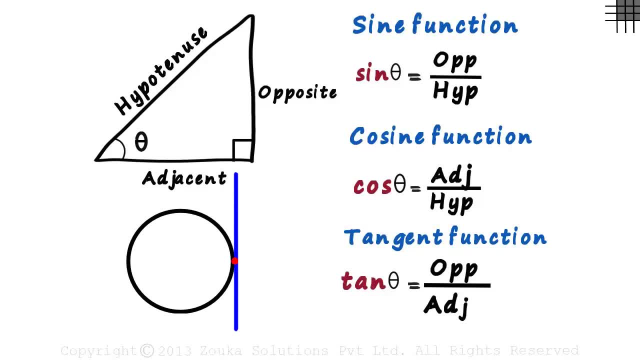 Isn't it a line which meets the circle at just one point? Yes, that's correct, But we don't see a line or a circle anywhere in the picture. Don't worry about it now. You will know why it's tangent in one of our other videos. 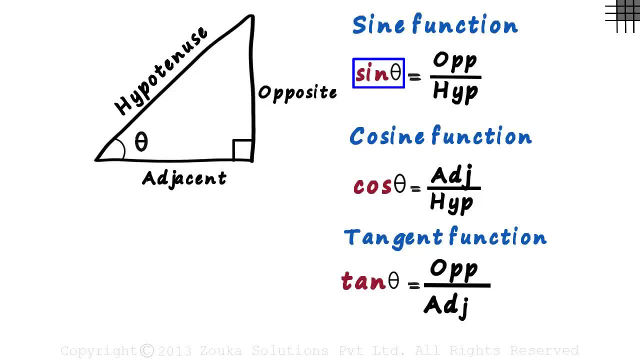 So let us review what we just did. Sine theta is opposite by hypotenuse, Cos theta is adjacent by hypotenuse And tan theta is opposite by adjacent. Let's play with these formulae. Let's try dividing sine theta by cos theta. 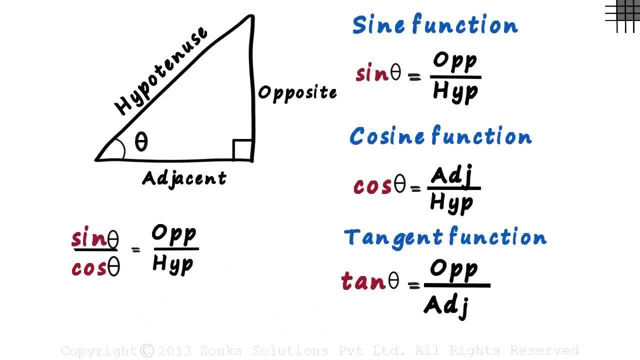 Sine theta is opposite by hypotenuse. Sine theta by cos theta also equals sine theta multiplied by one by cos theta. One by cos theta is actually the reciprocal of cos theta, And the reciprocal of cos theta would be hypotenuse by adjacent. 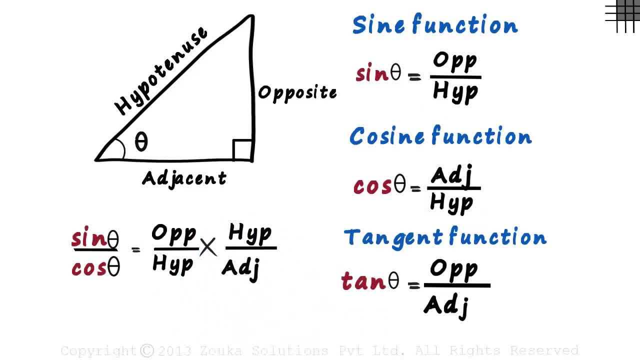 So we multiply this by hypotenuse, by adjacent. Look at the right hand side. Can we reduce it further? Yes, we can cancel out hypotenuse from the numerator and the denominator. That gives us opposite by adjacent. Hang on, does this look familiar? 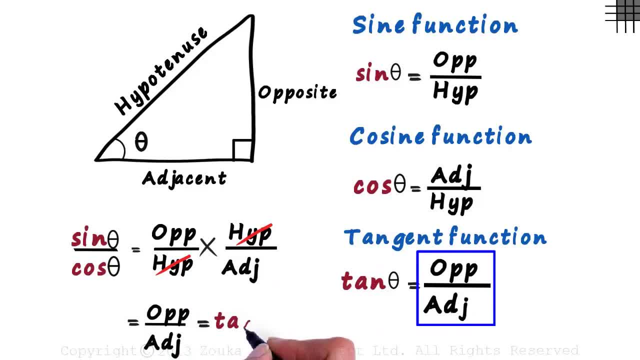 Of course it does. It's the value of tan theta. We just proved one of the most important relations in trigonometry: Sine theta by cos theta equals tan theta. But how do we remember so many formulae? It's very simple. 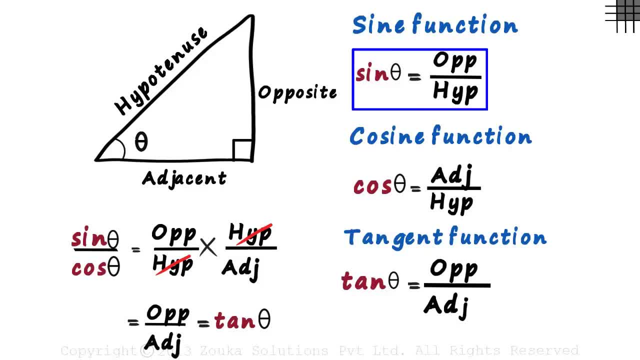 Observe the first letters in each of the cases. Look at the first formula: S, O and H. So let's write SOH here. Now look at the second formula: It's CA and H, So we write CAH here next to SOH. 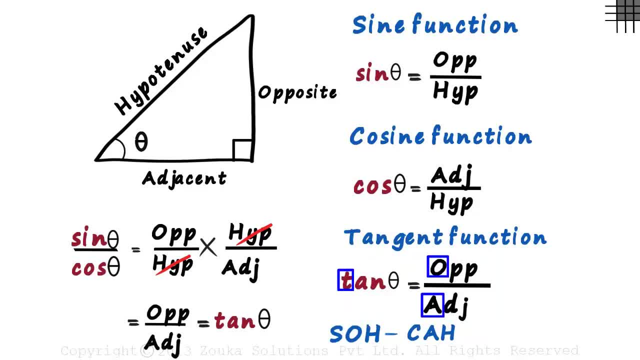 And in the third formula it's TO and A. We write TOA here. What we get is SOH CAH THWA. Well, it may sound funny, but that's the best way to remember the formulae: SOH CAH THWA. 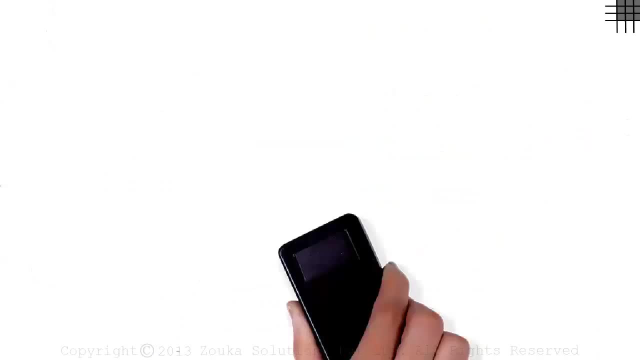 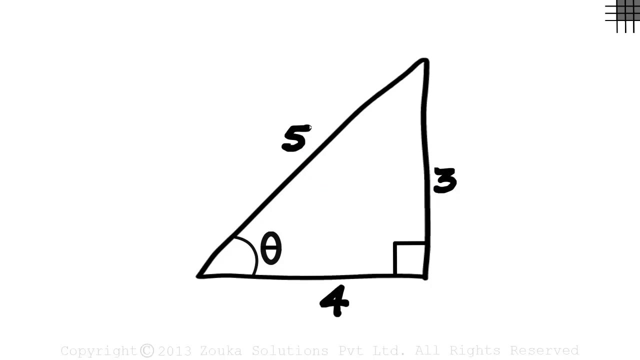 So let's review the formulae one last time in this video. Assume we have a right triangle with lengths 3,, 4 and 5 units. Before we find the values of sine, cos and tan, let's write our code on top.